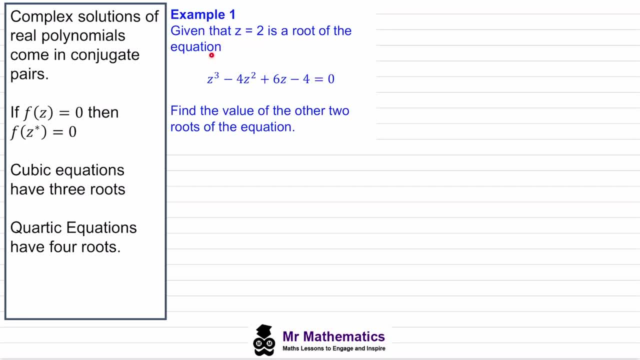 we're given that z equals two is a root of this cubic equation, and you can see that this is a real root. We've been asked to find the value of the other two roots of the equation. So if we say, then, that the function of z is equal to z cubed minus four, z squared plus six, z minus four. 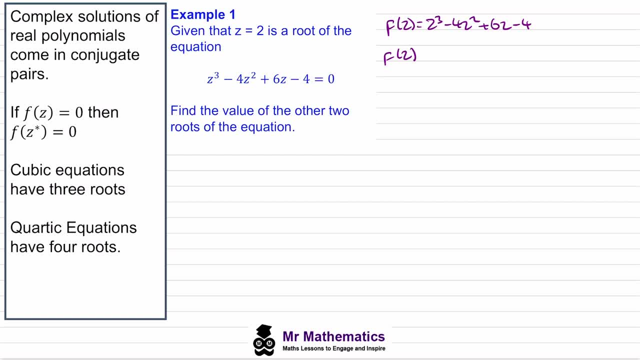 then we know that f of two, when z equals two, is equal to zero. So therefore z minus two, using the factor theorem, must be a factor, And if this is a factor, we can use long division to find the quadratic factor. So now we'll divide. 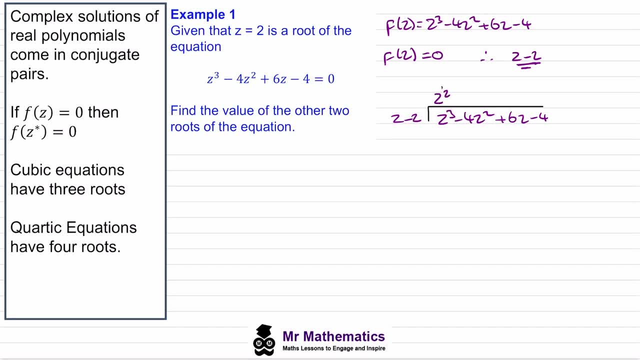 the z cubed by z squared, And we get z squared. We'll multiply this out and we get z cubed minus two z squared. The difference in our quadratic terms is negative two z squared. We'll drop down our linear and our constant. Then we'll divide this negative two z squared by 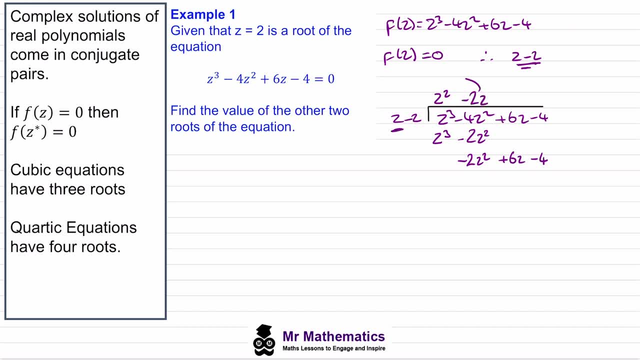 this z, So we get negative two z. Then we'll multiply it out again, So negative two z squared plus two z squared Plus four z. These will cancel, and then the six z take away from four z will give us two z. 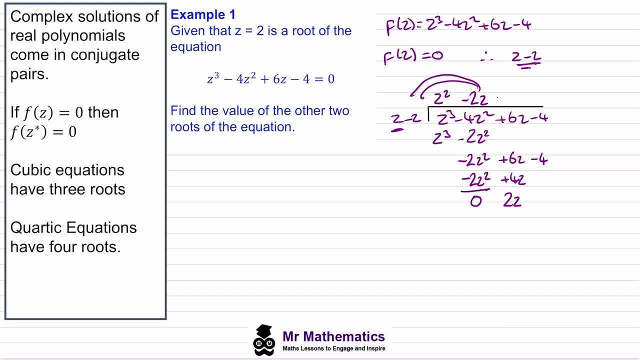 We'll divide this by z and we get positive two. We'll drop down the constant, mean negative four and then we'll multiply this out again, So two z minus four. okay, So we know our quadratic factor will be z squared minus four, z squared. 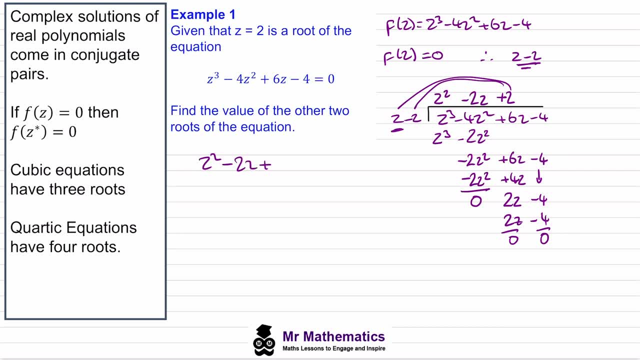 squared minus 2z plus 2, and this will equal 0.. So now to find the other two factors. we need to solve this equation and I'm going to use the method of completing the square. So we'll half the negative 2. we get z minus 1. we'll square this, we'll complete the square, then we'll add back in. 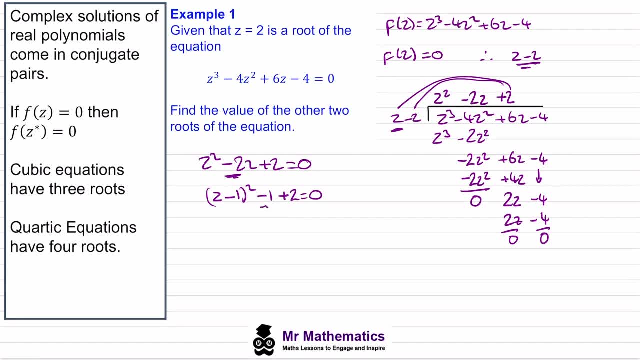 with 2 we'll move this positive 1 to the right hand side, so z minus 1 will equal negative 1. so we get z minus 1 will equal plus or minus the square root of negative 1.. We know that the root of negative 1 is i and we can move this negative 1 to the right hand side, so we get z is equal to. 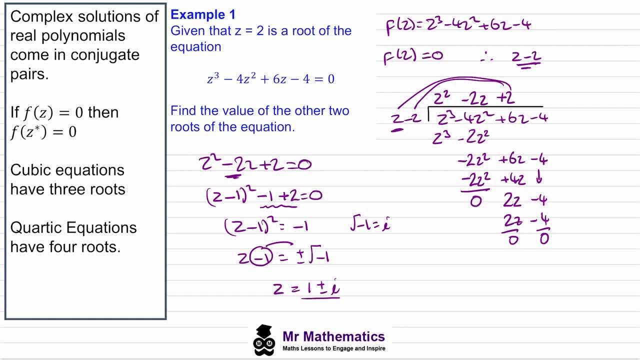 positive 1 plus or minus i, Then these would form our other two roots, our complex roots. So we know then that, in total, the three roots are: z is equal to 2 and z is equal to 1 plus i and its complex conjugate. 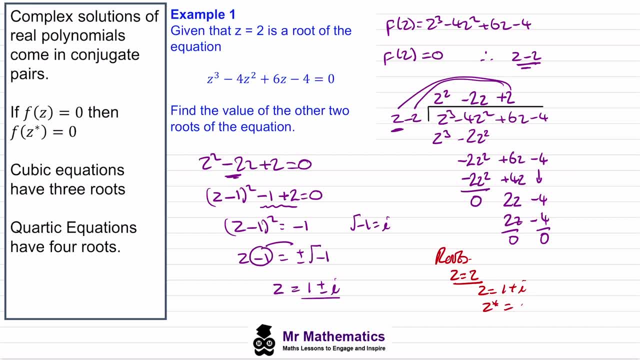 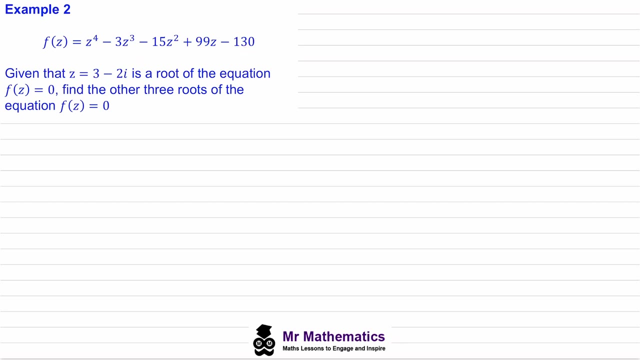 then star is equal to 1 minus i. Okay, so I hope this has given you an idea on how to find the complex roots of cubic equations. In example 2 we're going to look at a quantic equation, Okay. so in example 2 we're told that f of z is this quantic equation and we're given that z 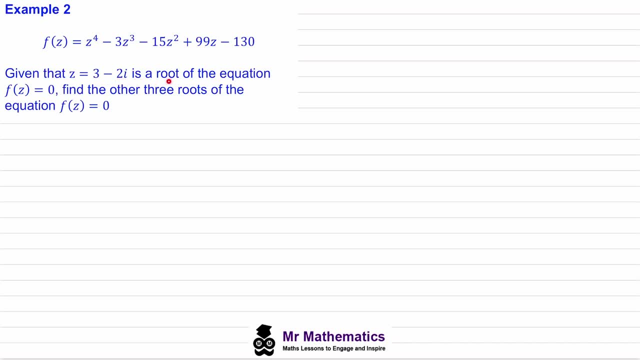 is equal to 3 minus 2i is a root of the equation where f of z is equal to 0, and we've been asked to find the other three roots of this equation. So if we go back to what we said earlier, in that 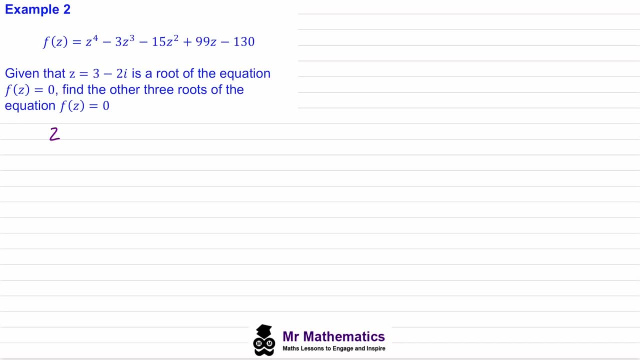 the roots occur in complex pairs. We know z1 is 3 minus 2i and z2 will be the complex conjugate of z1, 3 plus 2i. And now we can use these two roots to find the quadratic factor of this quantic equation. 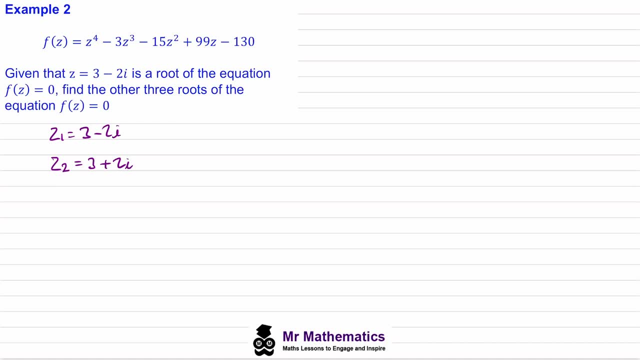 If you remember from a previous video looking at quadratic roots, well, if we've got roots- alpha and beta- in this case z is equal to 1 minus 2i- Then we can write a quadratic as z minus alpha, multiplied by z minus beta, is equal to 0 and we 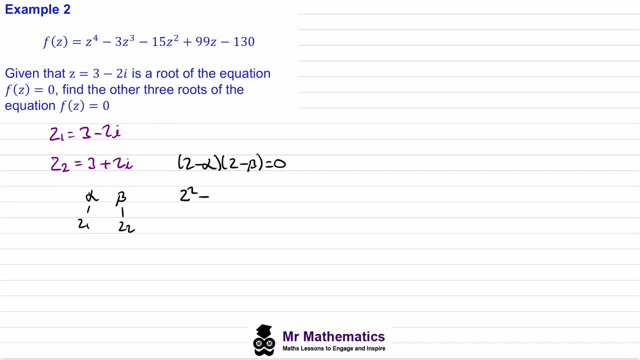 can expand this out. so z squared minus alpha plus beta plus alpha beta. sorry, z plus alpha beta will equal 0.. So we can work out the quadratic factor By adding these two roots together to work out this term and multiplying them together to work out the constant term. 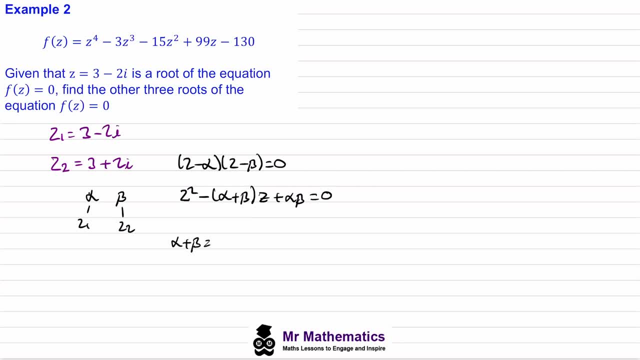 So alpha plus beta will be z1 plus z2 plus 3 minus 2i plus 3 plus 2i. the two i's will cancel. So alpha plus beta will be 6, and then the constant term alpha beta will be the product of the своих equationwon't cancelin the root of the equation. 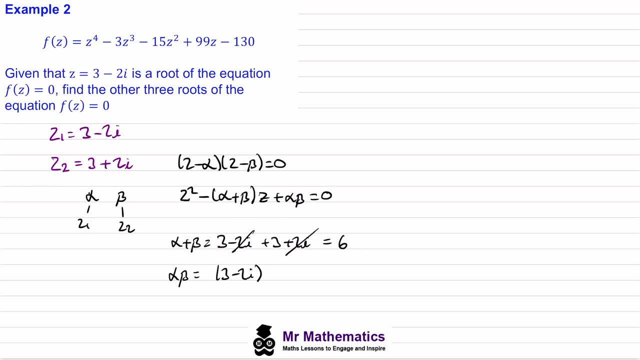 roots. so 3 minus 2i multiplied by 3 plus 2i- we can expand this out- we get 3 times 3, which is 9, and then we get the negative 2i times positive 2i, which would be negative 4i squared. 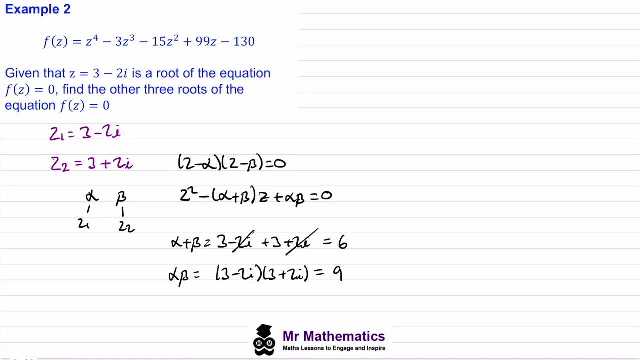 which we know is negative 4 times negative 1, so plus 4, so this would be 13.. so what this tells us, then, is that our quadratic factor will be z squared minus 6z plus 13. and this will equal zero. so this is our first quadratic factor, and we can use the method of. 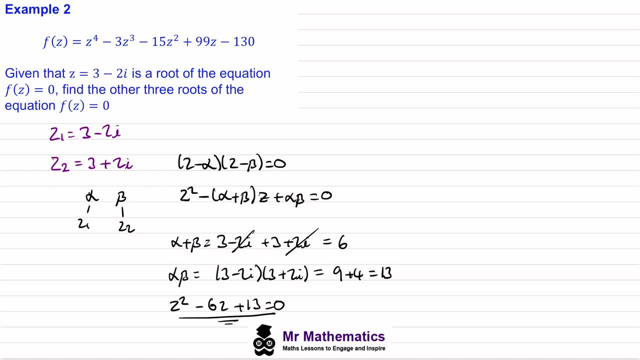 equating terms to find our second quadratic factor. so we know z squared minus six, z plus 13 multiplied by another quadratic. so in its general form, a, z squared plus b, z plus c, will be equal to our quartic. z to the four minus three, z cubed minus 15, z squared. 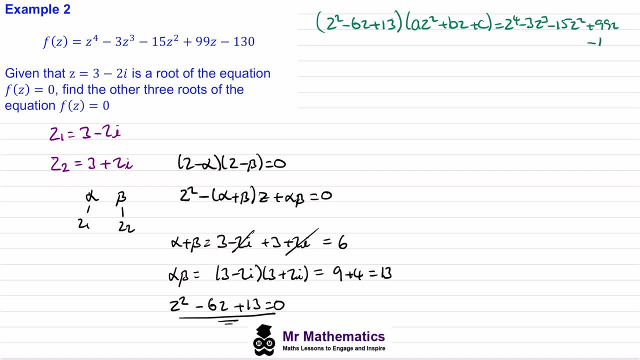 plus 99, z minus 130.. okay, so now we can equate terms. we know this z to the four we can only get by multiplying z squared by this, a z squared, so a times z to the four, we know, must be equal to z to the four. we can cancel out the z to the fours. so, in order, a must be equal to one. 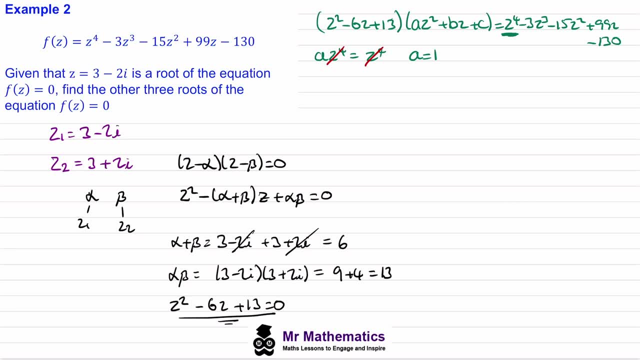 our cubic term. we can only get for multiplying the z squared by the z and this a z squared by negative six z. so negative six a z cubed plus z squared multiplied by b z. so b z cubed must equal negative three z cubed. we'll cancel out the z cubes and we know that a is one. so